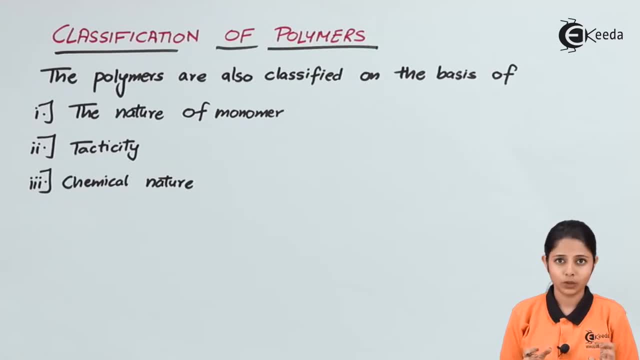 macro means huge. So where, if I am talking about micro, that means those are small molecules. Whenever I am talking about macro, that means those are huge molecules. These macromolecules have high molecular weights. So when macromolecules- that means huge molecules with high molecular weights- come together, when all of them come together, they form something. 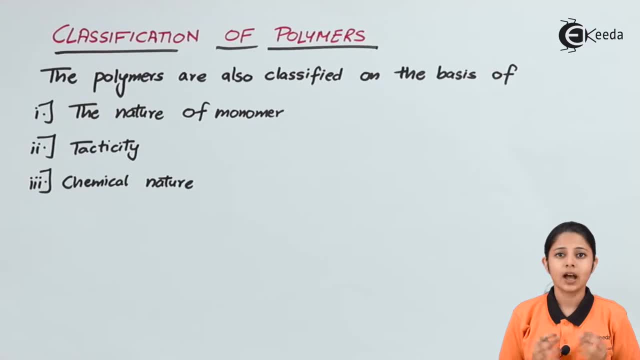 known as polymer, And these polymers are being used in various household, domestic as well as industrial appliances everywhere. Let us study their classifications in detail. The polymers are classified on the basis of: the first is the nature of the monomer? Now it depends. 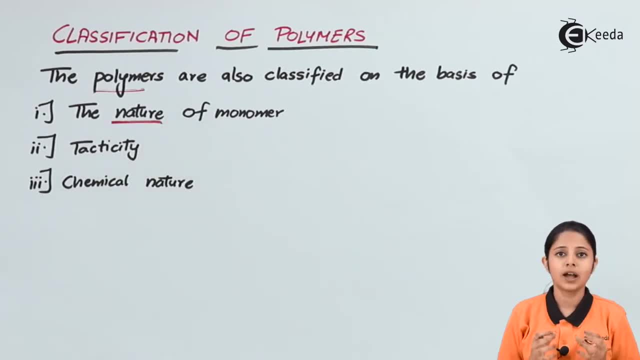 on the nature of the monomer. So monomer itself is a high molecular weight macromolecule and many monomers come together to form a polymer. Now this monomer has different kind of natures. Now, what exactly do we mean by nature? Nature is nothing but the properties, The 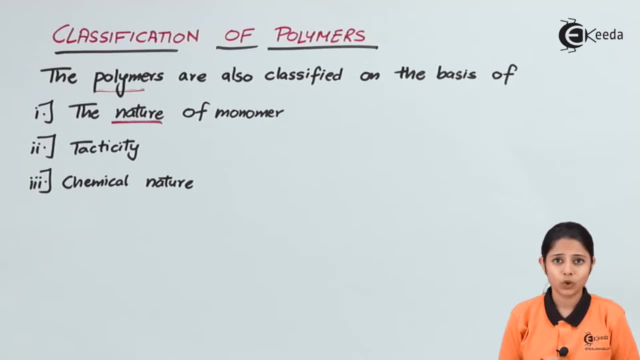 physical properties, the chemical properties, whether that monomer is organic or inorganic. all of that depends on nature, on the nature of the monomer, and the polymers can be classified on that. the second over here is the tacticity. tacticity is nothing but a stereochemical arrangement of polymers. 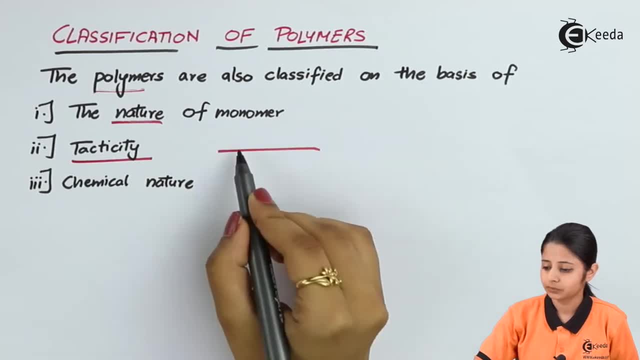 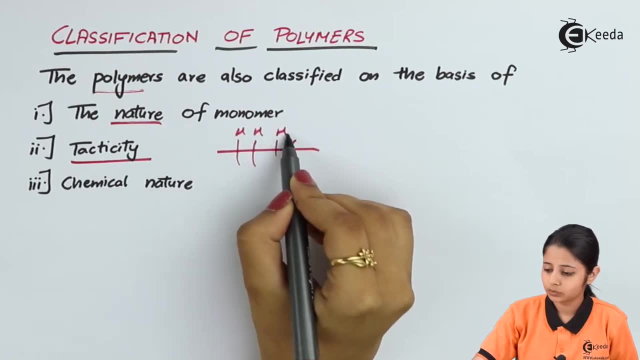 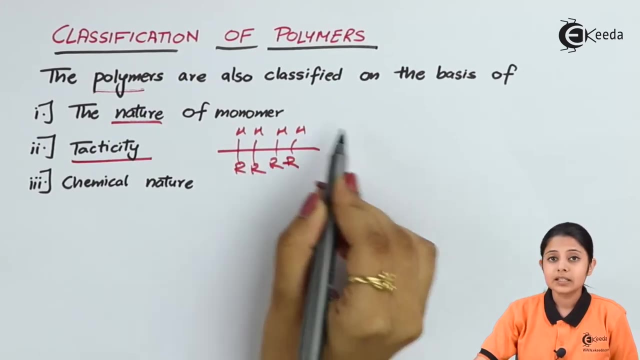 so, for example, if i have polymers over here and all the hydrogens are present above and all the alkyl chains are present below, this is nothing but an arrangement. this is nothing but a stereochemical arrangement. stereo means position, and chemical means all the elements which are present in it. 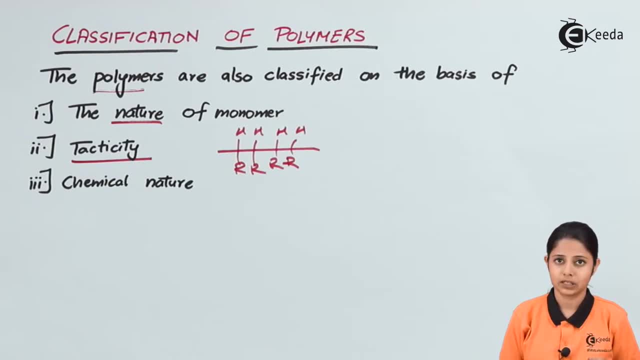 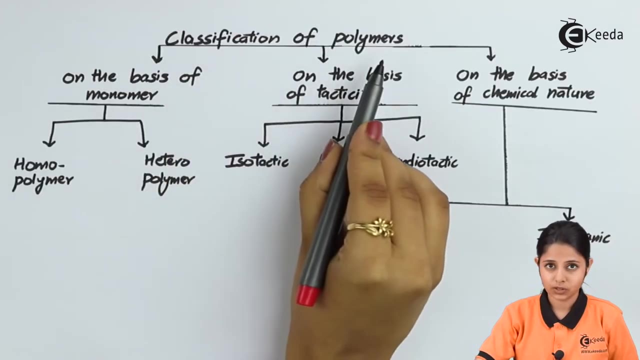 so based on the positioning also, polymers can be classified. and the last is the chemical nature, whether it is reactive, not reactive, whether it's a homopolymer or a heteropolymer. we'll come and see all these terms in detail over here. classification of polymers. 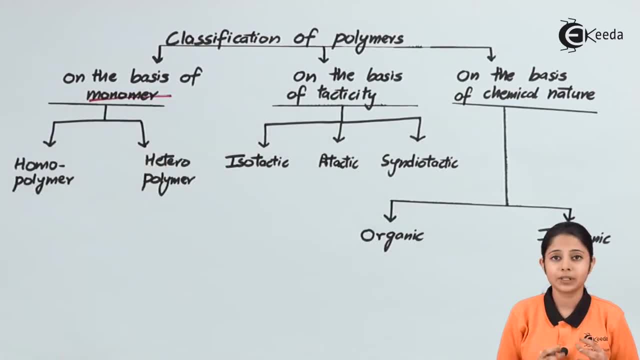 so this is the classification of polymers. the first is on the basis of monomer. monomer is nothing but the macromolecule, that is, the high molecular weight, huge molecule which come up together and form a polymer. now this monomers can be classified as homopolymers or heteropolymers. 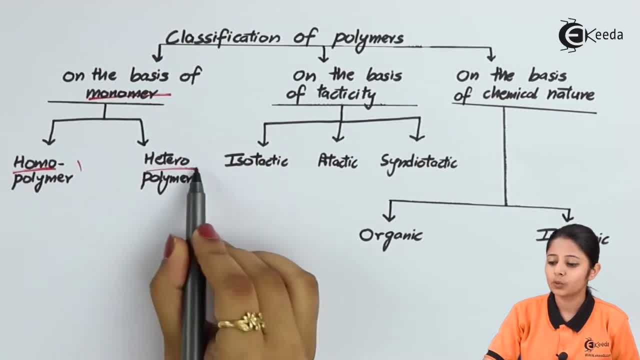 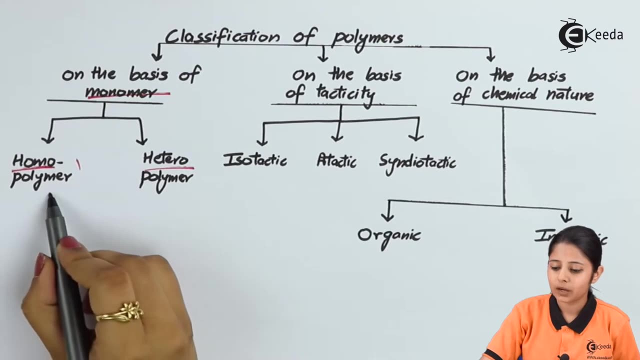 homo means one phase, hetero means many phases, homo means just one. so, for example, if i have ethylene, that is polythene, polythene bags. polythene bags are those bags which we use for carrying vegetables, fruits etc. they are just made up of carbon, so they are carbon to carbon chains. they may have. 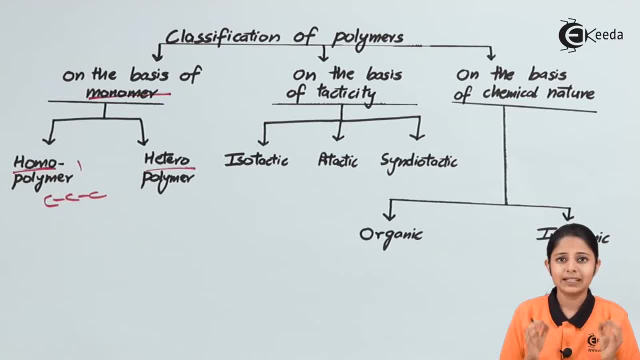 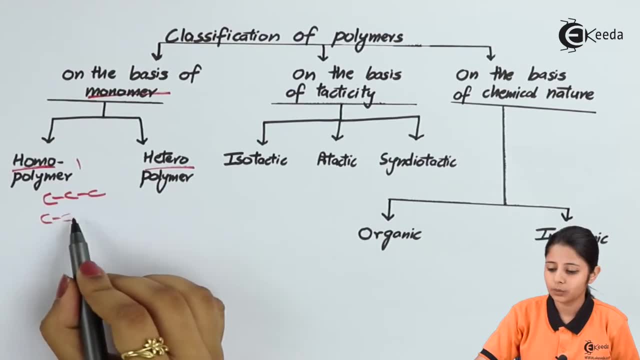 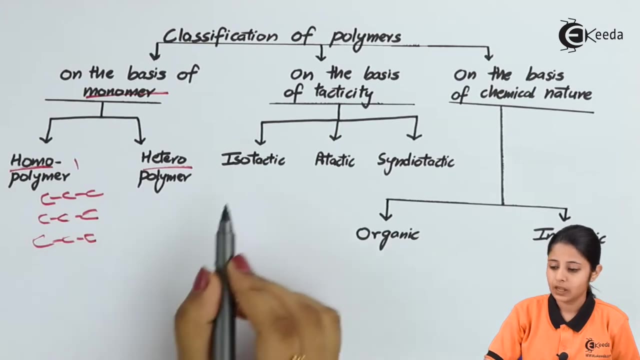 certain amount of hydrogen also present in it, but mainly it is carbon. those are known as homopolymers. now to these carbon chains. so this is nothing but my homopolymer. giving an example of polythene, this is a homopolymer. when i'm talking about heteropolymer, i'll give the same example that. 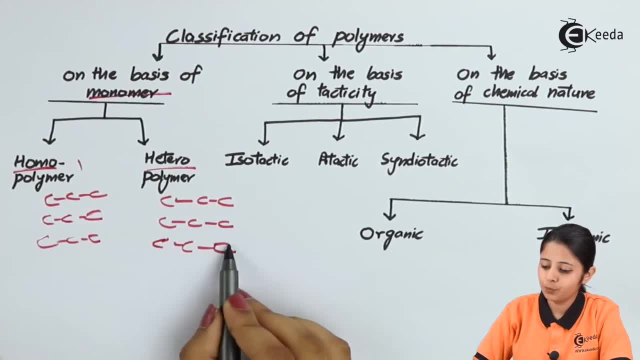 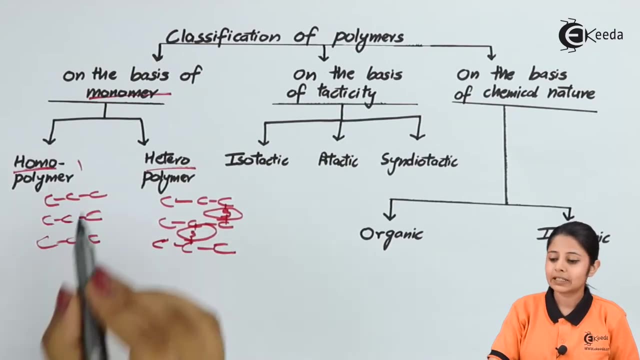 is, we have a linear chain of carbon over here, but now between these carbons there can be sulfur. that means a chain of sulfur in the middle. this can be possible and because of this sulfur linkage it will become a heteropolymer. this is the difference between a homopolymer and a heteropolymer. 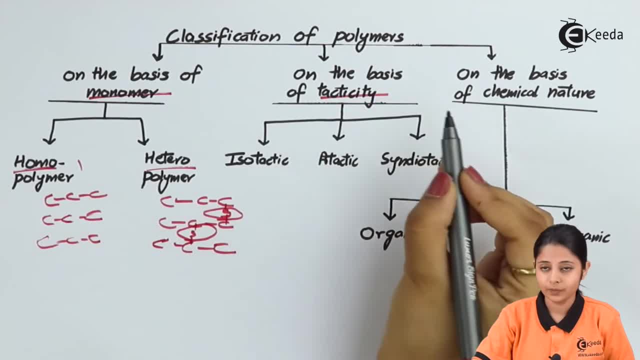 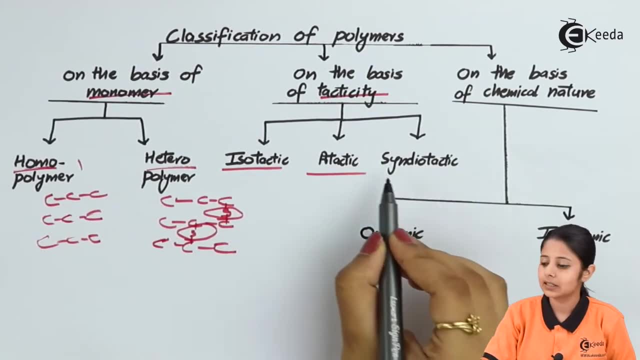 the second classification is on the basis of tacticity, and on the basis of tacticity it can be considered as isotactic, a tacticic tactic and syndiotactic. So over here let us see an example of isotactic. If I have a polymer over 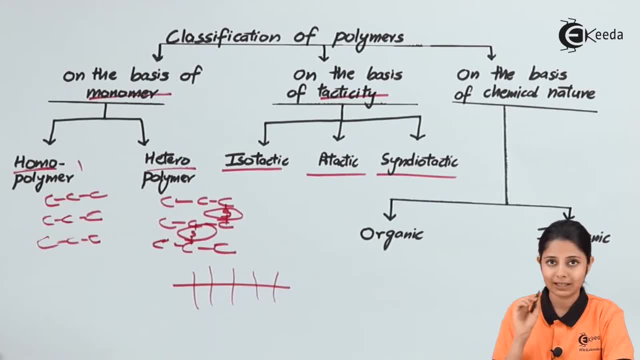 here. this polymer is made up of two things: R's and H, where R stands for any alkyl group- Alkyl group is any group containing carbon- and H stands for hydrogen. So if I have hydrogen over here on all the parts which are above and R over here on all the parts which are below, 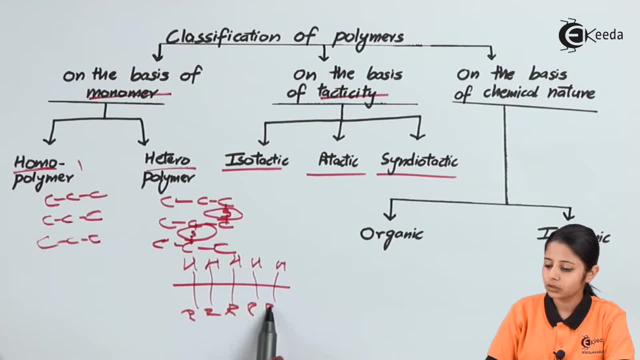 This is an example of isotactic. When I am talking about atactic, what happens is the R's and the H's may fumble. that means they may go from one place to another place, but there will be some kind of pattern over here. So, for example, if I take this R H, R H, that means the R's are. 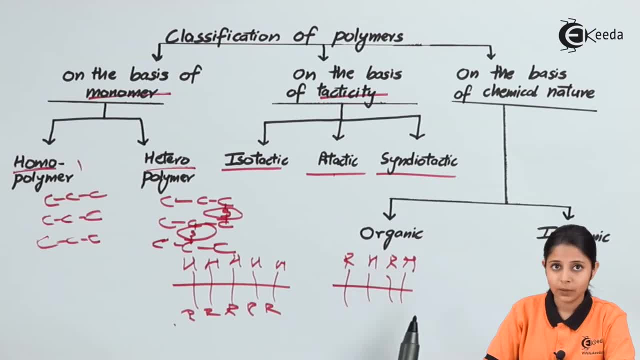 on above. the H's are also above this line, But now they are following an alternate pattern. So R then one H, then one R then one H. This is nothing but my pattern. This is known as atactic. Finally, we have syndiotactic. This also has some 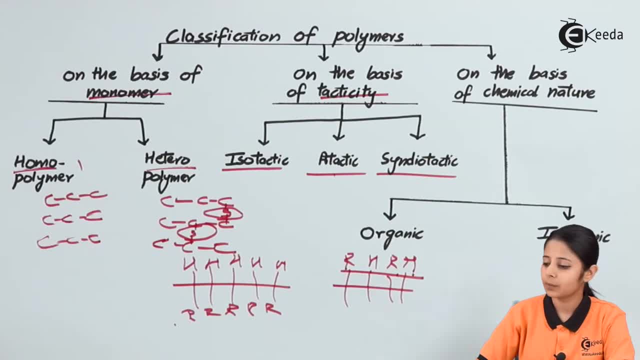 pattern, but this won't be an alternate pattern. For example, if I have one R, then I will have three H's, then my next R. This is nothing but my pattern. This is known as atactic. Finally, we have syndiotactic. This also. 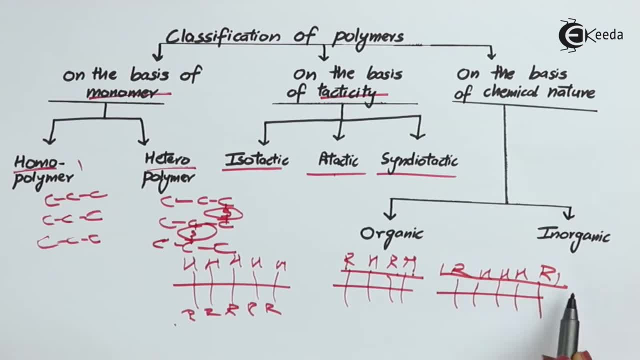 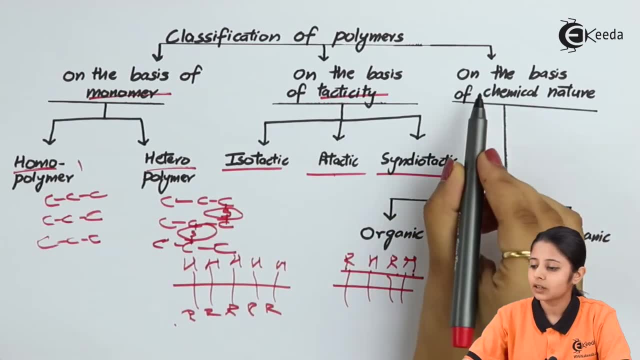 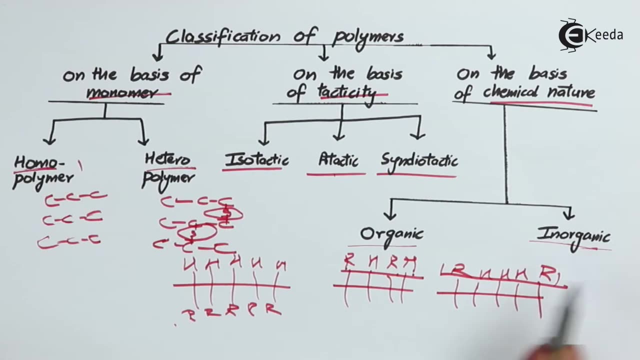 is nothing but a pattern over here, where one R H, H H, another R. This is known as a syndiotactic. So these are based on the tacticity. The third kind over here is on the basis of chemical nature. This can be organic or inorganic. What do we mean by organic? Organic components? or organic compounds, or those compounds which are made up of hydrocarbons. Now, what are hydrocarbons? Hydrocarbons are nothing but substances which are made up of two things: Hydrocarbons and hydrocarbons are something very similar. Hydrocarbons are nothing but. 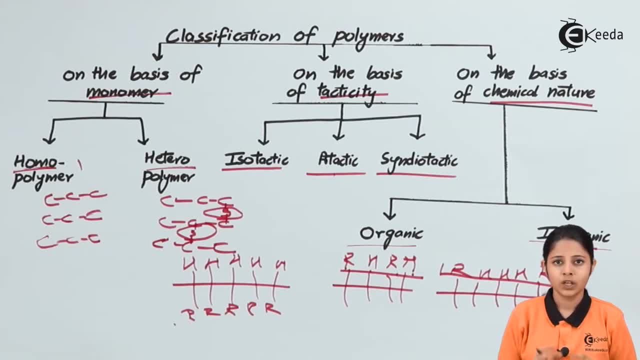 substances which are made up of two things: Hydrocarbons. and hydrocarbons are substances, two things: hydrogen and carbon. So when I have hydrogen and carbon with me, hydrogen and carbon together will form a hydrocarbon and that entire compound will be organic compound, Anything which 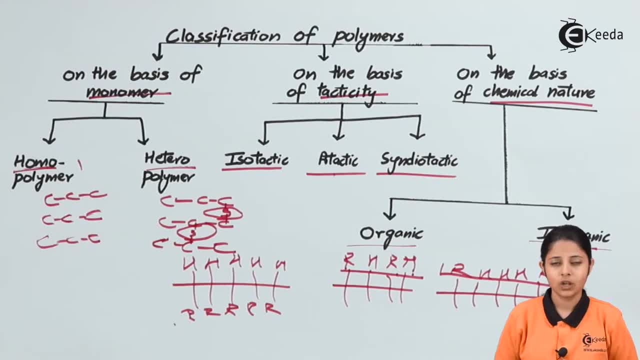 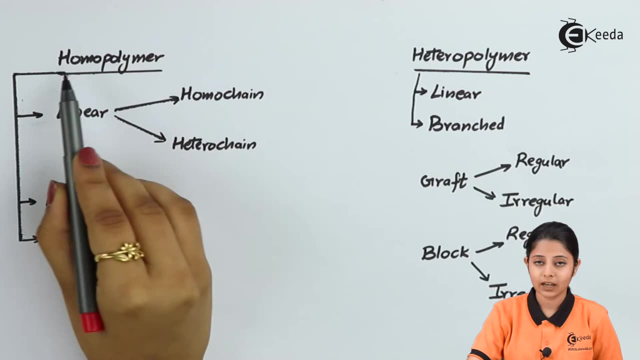 does not contain hydrogen and carbon are inorganic. Most of my natural polymers are organic in nature. There are many synthetic inorganic polymers as well, So here we are further classifying homopolymers and heteropolymers. Homopolymers can be classified into linear, branched or 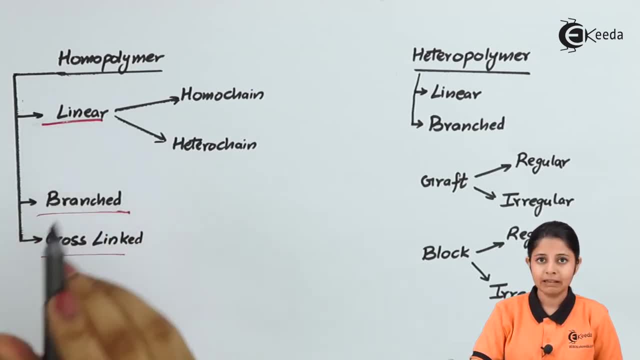 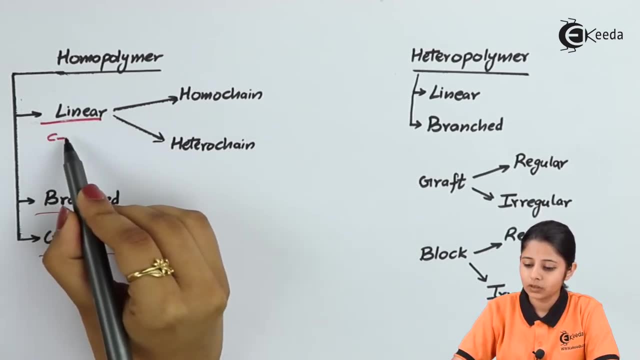 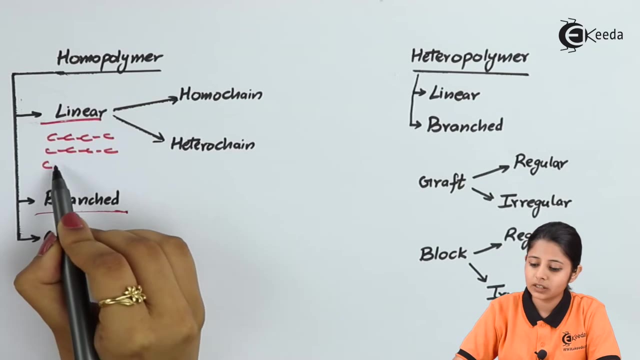 cross-linked. Now, what do we mean by linear? Linear is nothing but straight lines. So, for example, if I have carbon over here which forms straight chains, This is my linear polymer, because carbon is formed by heteropolymers. So if I have carbon over here which forms straight chains, 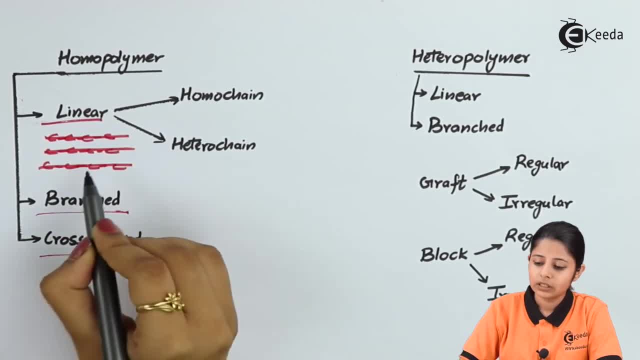 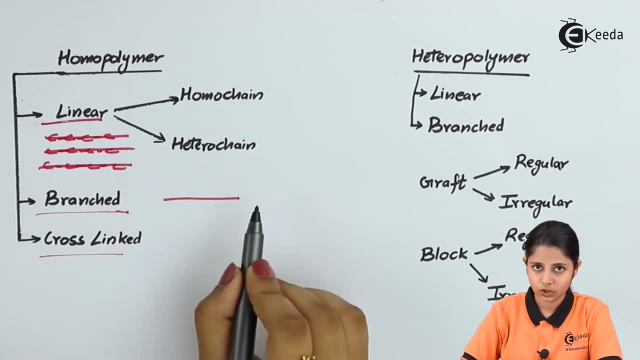 This is known as a linear polymer. What is a branched polymer? The carbon will form straight chains, but then there will be certain branches which will come out from here and there. This is known as my branched polymer. What is my cross-linked polymer? Cross-linked polymer also has linear 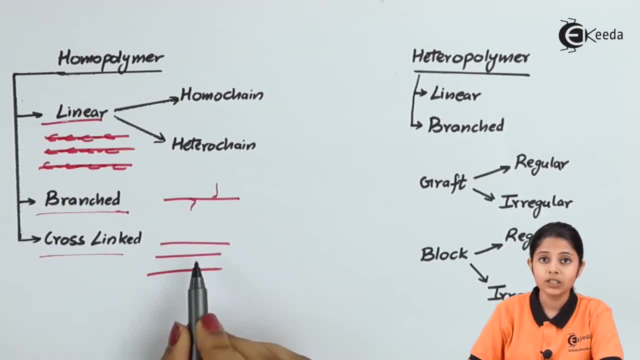 polymers. that means straight chain polymers, but all these chains are being linked By a cross-link. So, for example, if I have a carbon chain and between the carbon there is a sulfur which is linking two carbon linear chains, This entire polymer becomes my cross-linked polymer. 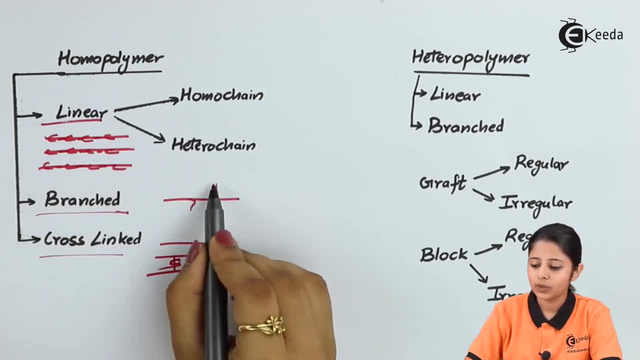 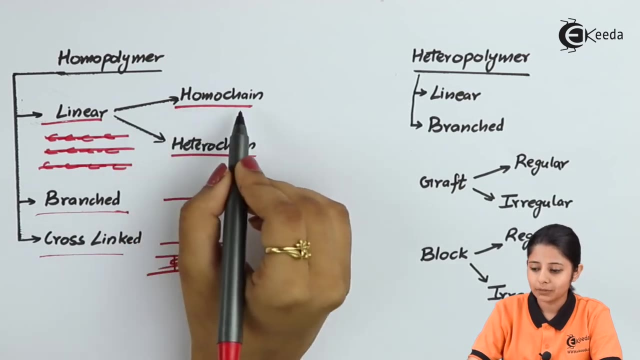 Linear polymers are straight chained, Branch are with certain branches and cross-linked are straight chain polymers, but there will be certain cross linkage between them. Linear polymers can be further classified into homo chain and hetero chain. Homo chain means all the chains will contain only carbon. So over here in this example of 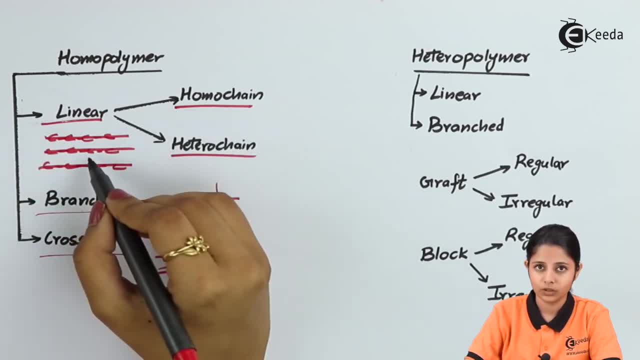 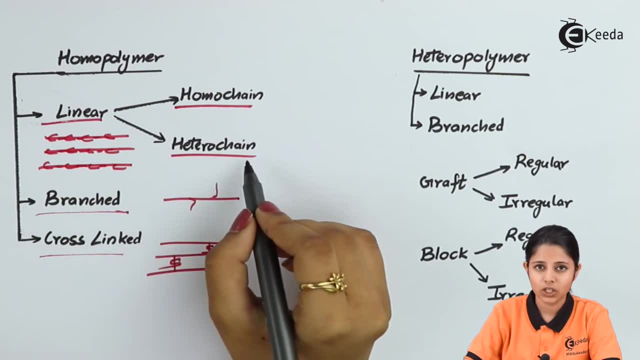 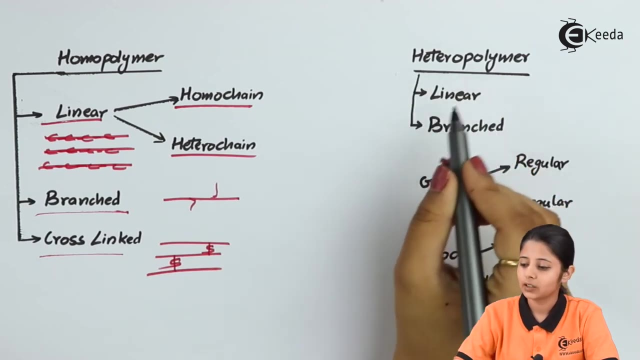 linear polymer. this is a homo chain linear polymer. Now why do we have it as a homo chain linear polymer? Because we only have carbon in it. There can be hetero chain as well. that means there will be different kinds of chains in it. Moving further to hetero polymers, Again hetero, 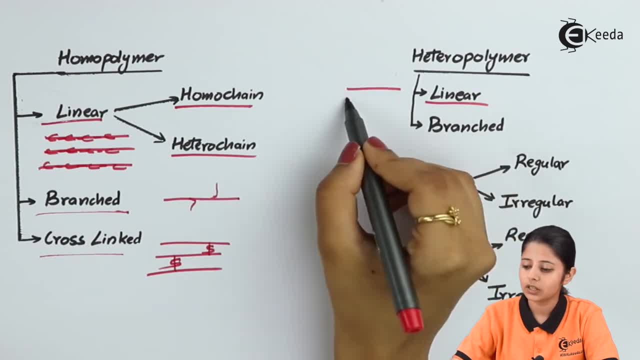 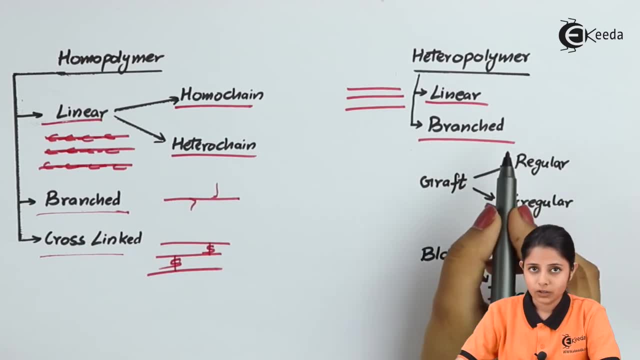 polymers are linear. that means straight lines. They are not interconnected. So if I have a carbon chain, it is not connected by any cross links or anything Next is branched. that means straight lines, but there will be a branch of something else. For example, if this is carbon, the entire. 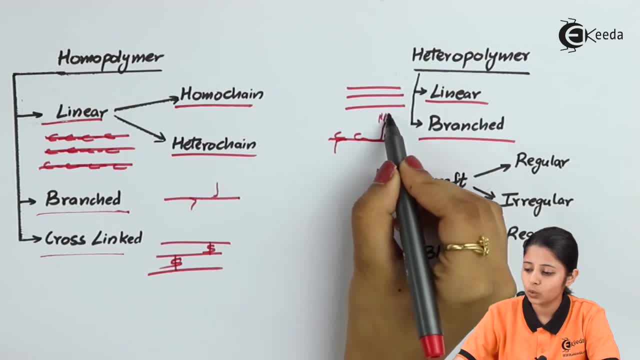 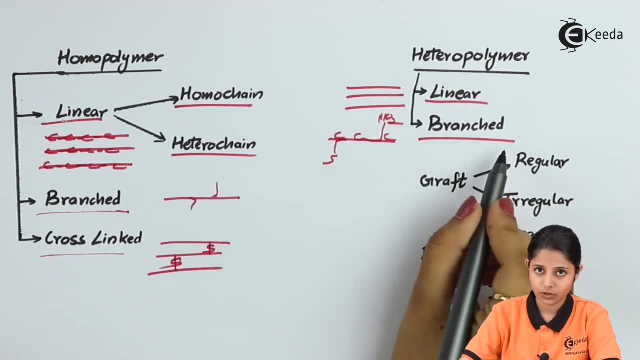 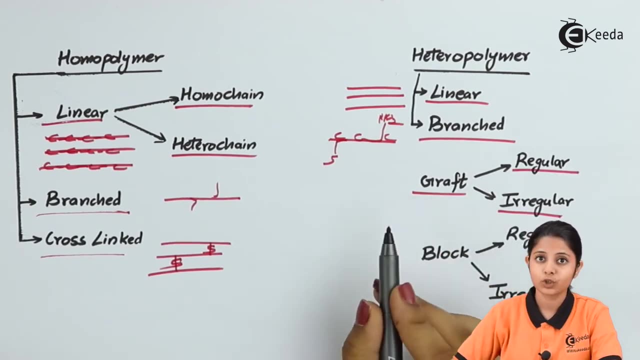 thing is carbon, but there is a branch of nitrogen or NO, nitrogas, NO2 over here, or we have something else like sulfur over here. This is nothing but branched. The next is graft. Now what exactly are graft polymers? Graft polymers are those polymers which have a strong backbone, So over. 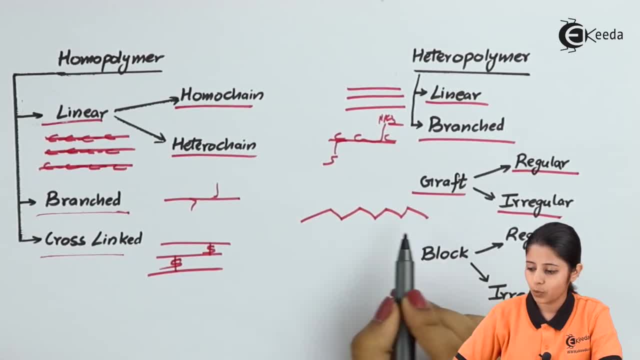 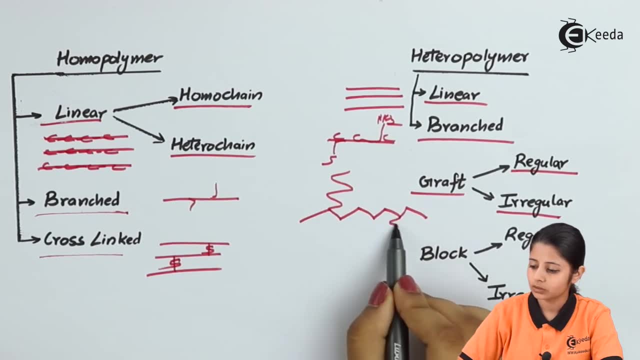 here. if I am drawing a graft polymer, this will be my graft polymer and this is the backbone of the polymer, and this backbone will have certain chains attached to it. For example, this backbone is made up of carbon, So all the points or the vertexes will be my carbon. All of these are carbon. that 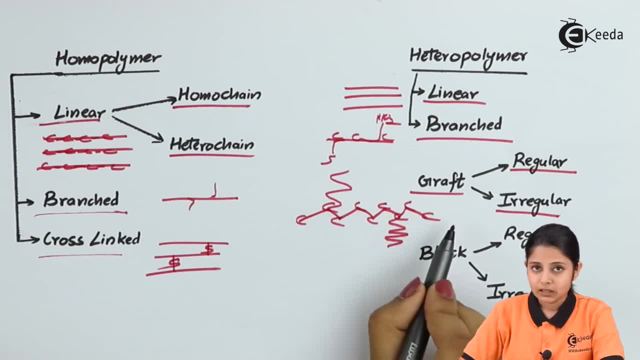 means my main backbone is carbon and this backbone will have certain branches attached to it. This is my graft polymer. If the branches are at regular intervals, it will be my regular graft hetero polymer. If these branches are not at regular intervals, it will be my irregular.